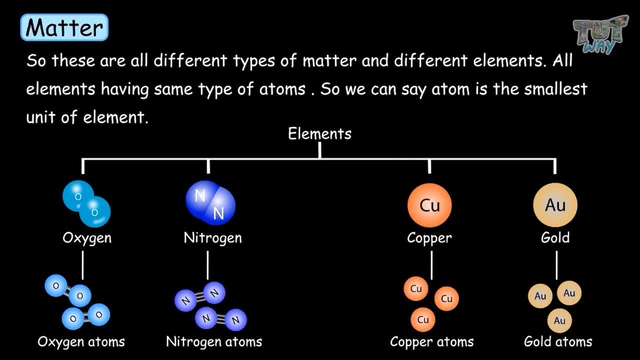 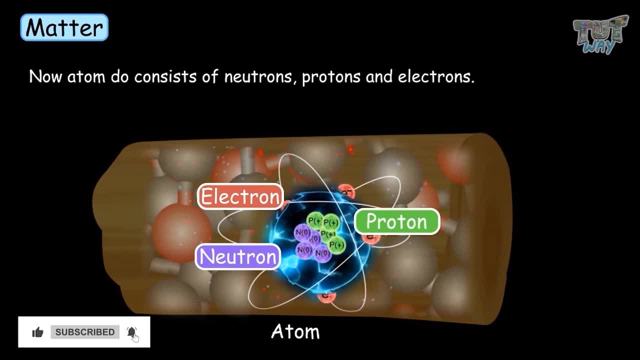 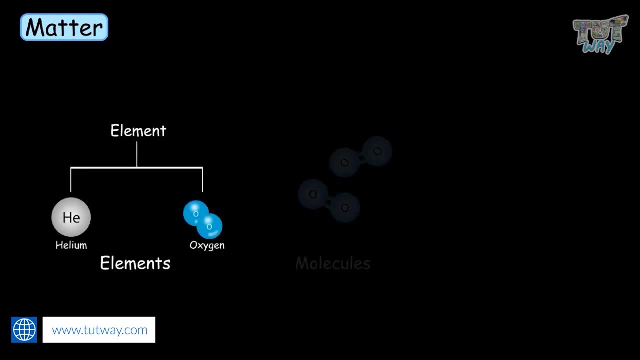 So we can say that the atom is the smallest unit of the element. Now, atoms consist of a nucleus, protons and neutrons, But we will see the detailed structure of the atom in our next section. Today we will learn about elements, molecules and compounds. 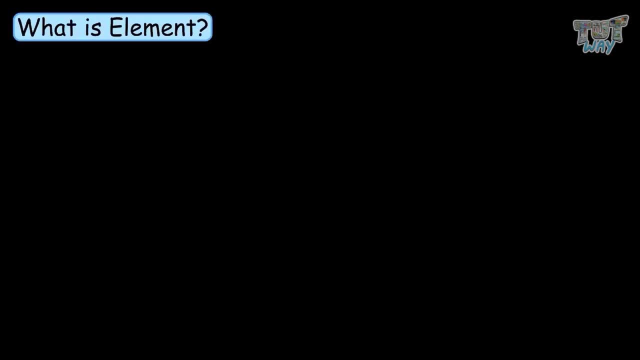 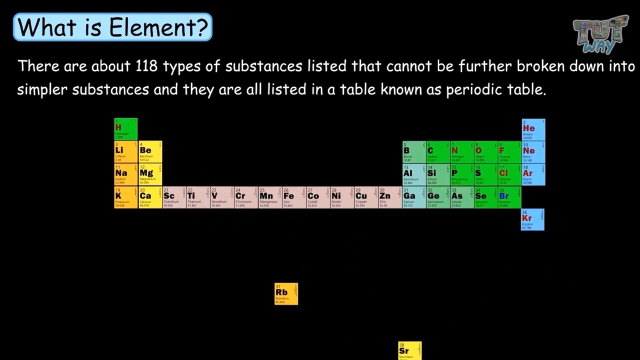 Now let's focus on what is an element. There are 118 types of substances listed that cannot be further broken down into simpler substances, And they are all listed in a table known as the Periodic Table As 118 types of different elements. This is the Periodic Table And 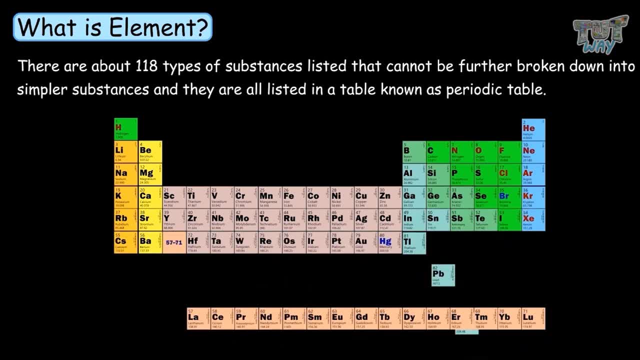 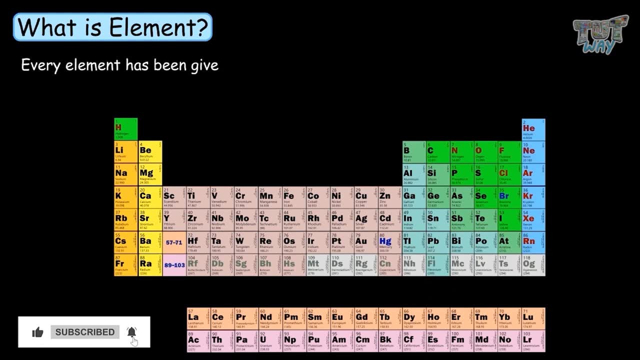 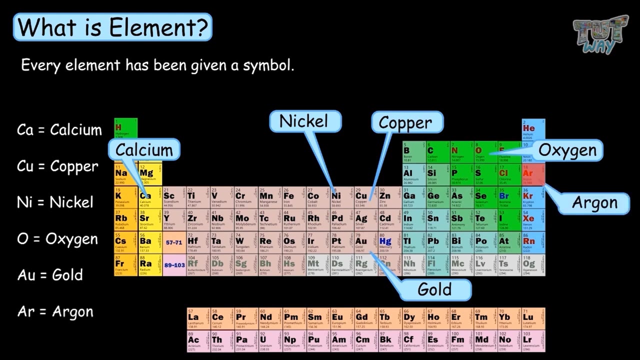 all 118 types of elements are distinct types of matter. They are listed in this table. Every element has been given a symbol. Ca stands for calcium, Cu stands for copper, Ni stands for nickel, O stands for oxygen. Au stands for gold, Ar stands for argon. 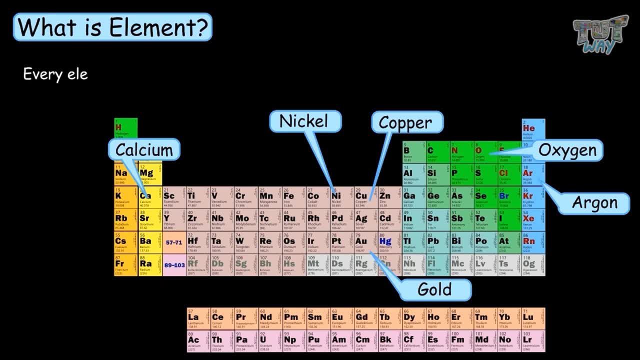 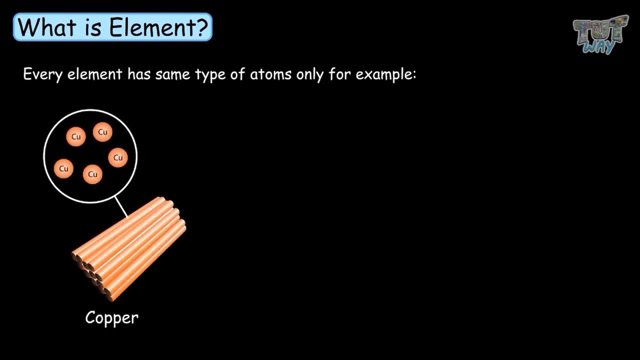 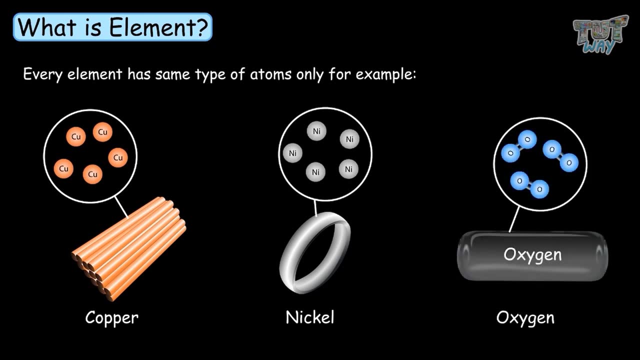 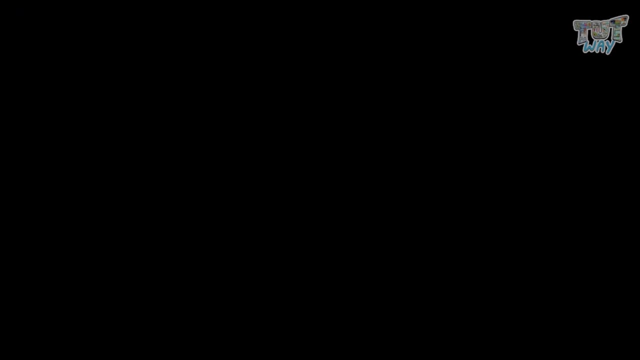 and so on and so forth. And every element has the same type of atoms only. For example, copper will only have copper atoms, nickel will only have nickel atoms, oxygen will only have oxygen atoms. So now we know what are elements. Now let's learn what are molecules. Let's take the example of oxygen. 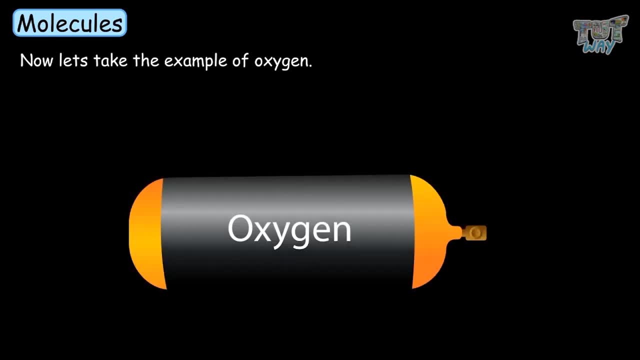 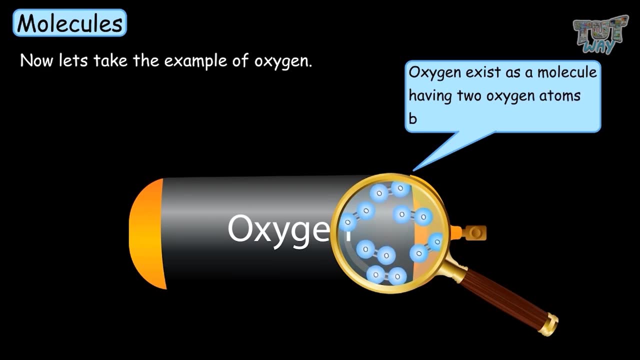 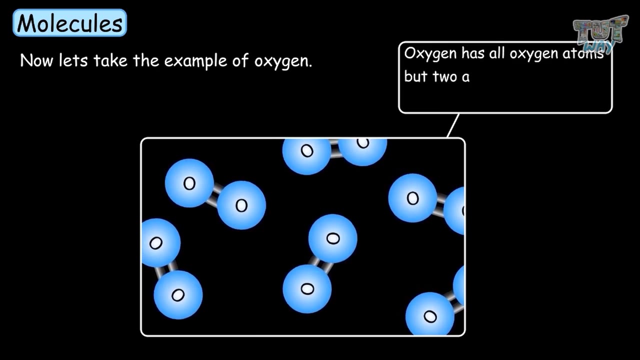 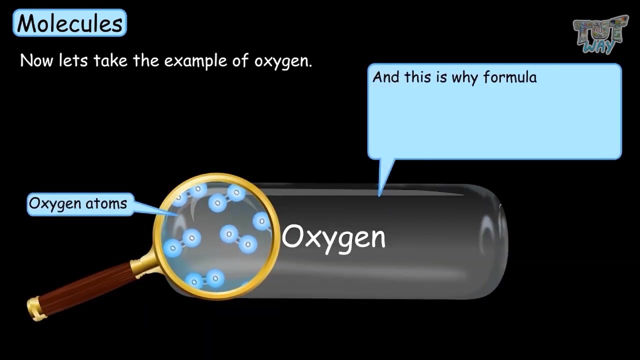 We learned that oxygen only has oxygen atoms. Now, in the case of oxygen, oxygen exists as a molecule That has two oxygen atoms bonded together, As in, oxygen is only oxygen atoms, but two atoms of oxygen are always bonded together, And this is why the formula of oxygen is O2, which means 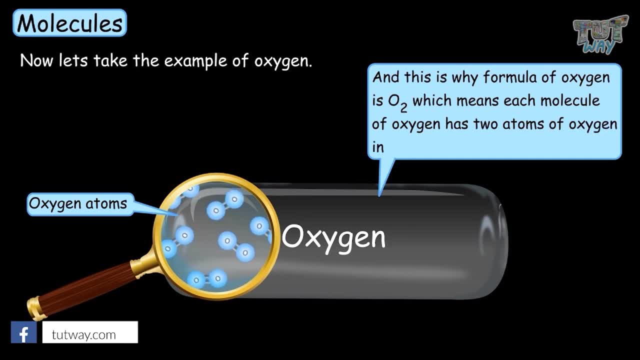 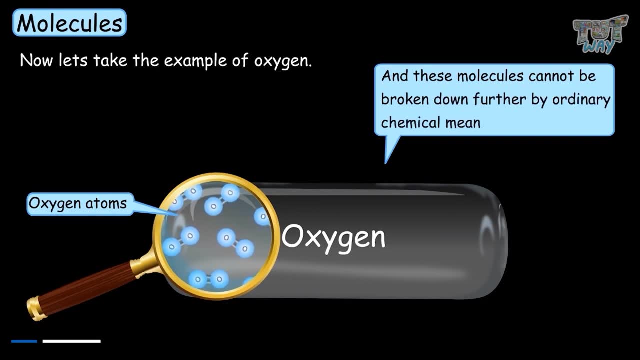 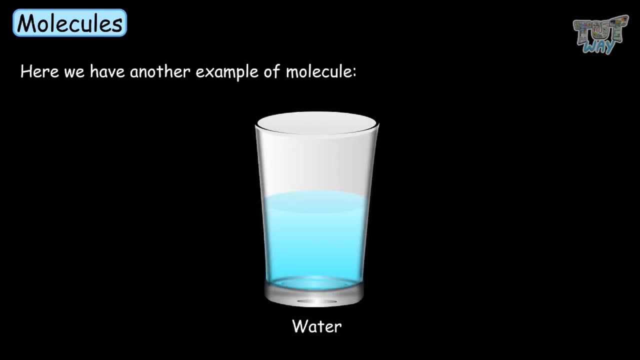 each molecule of oxygen has two atoms of oxygen in it, And these molecules cannot be further broken down by ordinary chemical means. Here we have another example of molecules: Water. Water is made up of two elements, oxygen and hydrogen, where water is molecules of water only, And each molecule is denoted as: 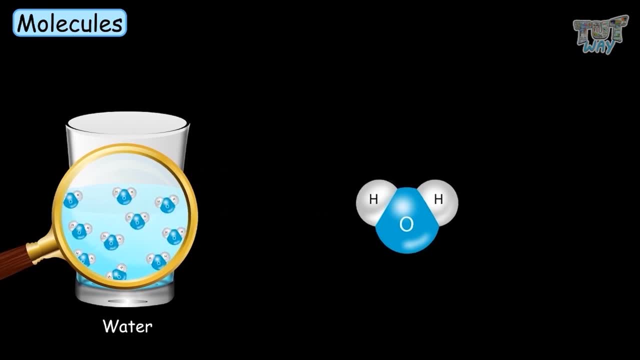 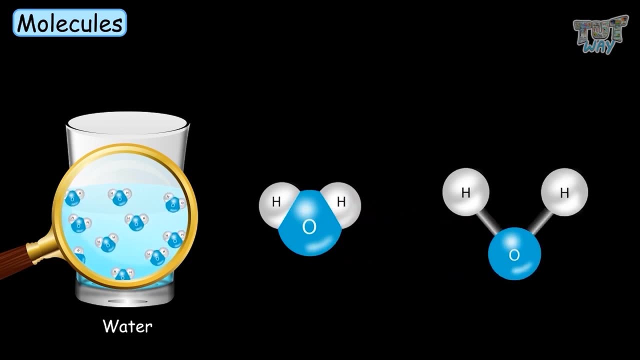 H2O, which means each water molecule has two atoms of hydrogen and one atom of oxygen. And that means that each molecule has two atoms of hydrogen and one atom of oxygen. You cannot further break down this molecule into atoms by ordinary chemical means. 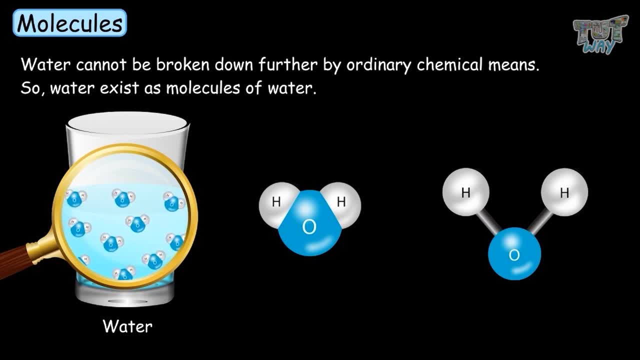 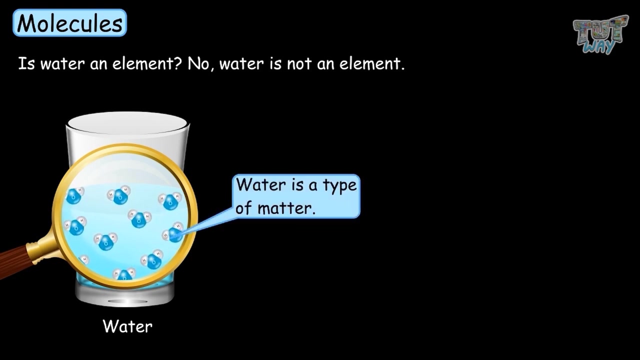 so water exists as molecules of water. Each molecule has two types of atoms: hydrogen and oxygen. Two types of hydrogen and one atom of oxygen. So is water an element? No, water is not an element. Water is a type of matter that has two types of elements: hydrogen and oxygen. 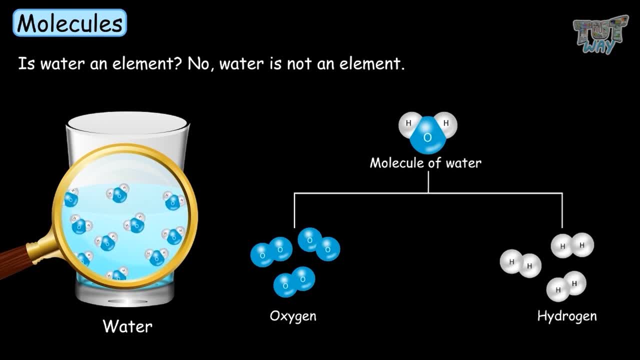 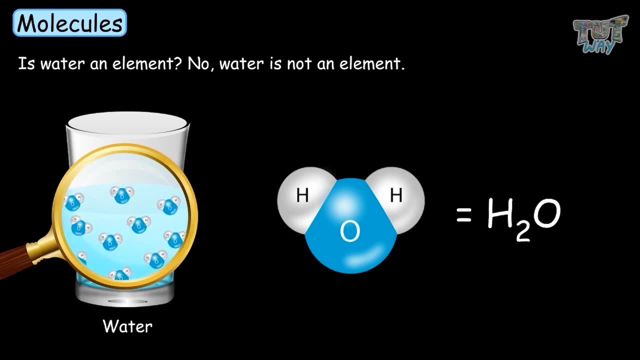 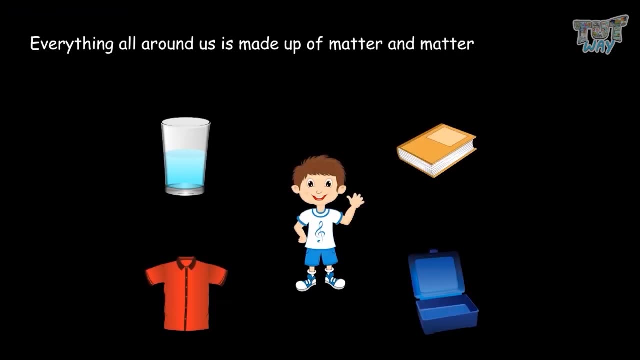 and they exist as molecules. Each molecule has the composition H2O. So let's revise it all again. Everything all around us is made up of matter, and, as you can see from what we've been describing, And matter is anything that occupies space and has mass. 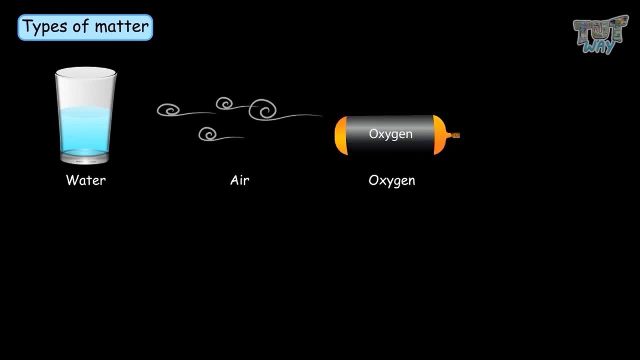 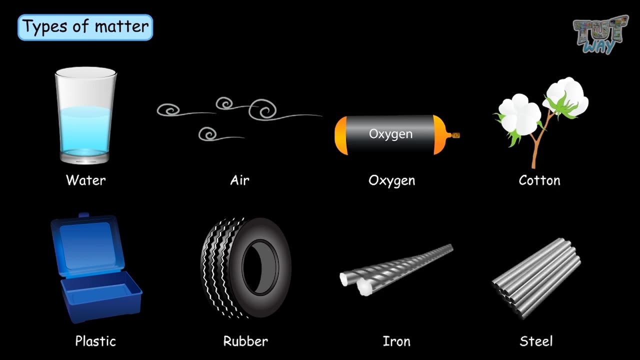 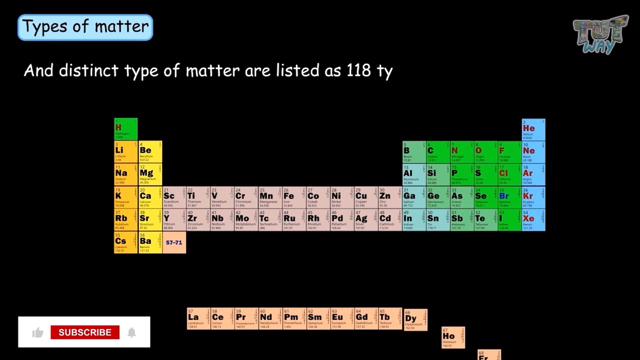 So water, air, oxygen, cotton, plastic, rubber, iron, steel. all of these are types of matter And distinct types of matter are listed as 118 types of elements And they are listed in the periodic table, And each element has a symbol. 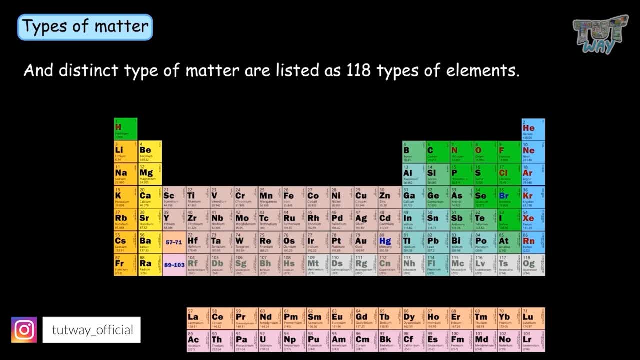 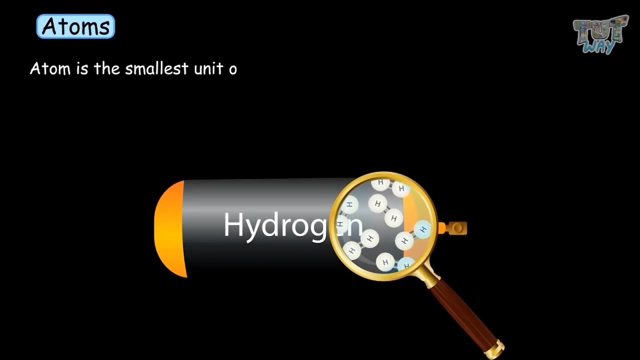 For example, hydrogen, oxygen, nickel, cadmium, silicon, helium. All of these are distinct types of matter As in these elements have the same types of atoms. So the atom is the smallest unit of matter. An atom exists as a molecule. 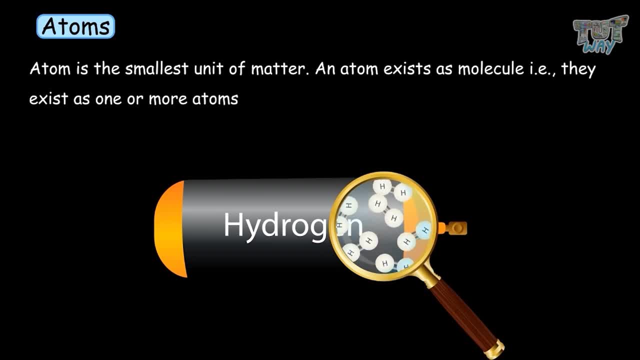 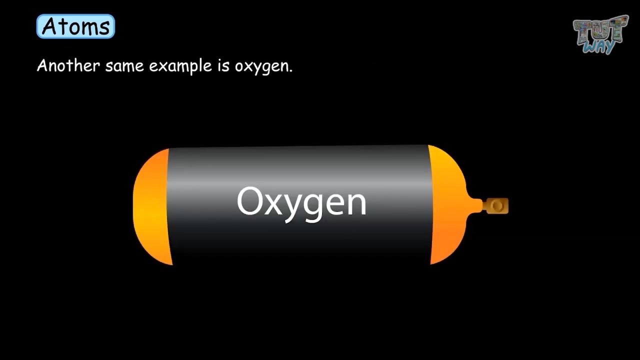 As in. they exist as one or more atoms bonded together, For example, hydrogen. Hydrogen exists as molecules of hydrogen, Where each molecule of hydrogen has two atoms of hydrogen bonded together. Another example is oxygen. Oxygen exists as molecules of oxygen, Where each molecule of oxygen has two atoms.